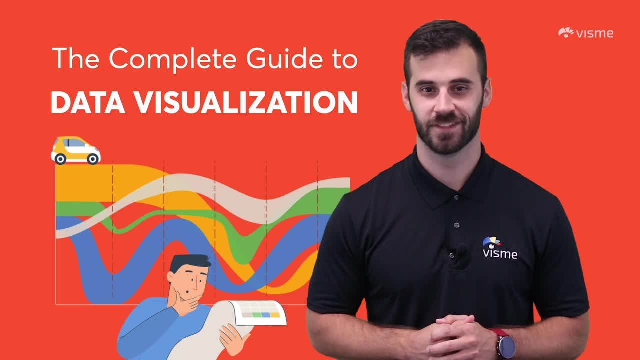 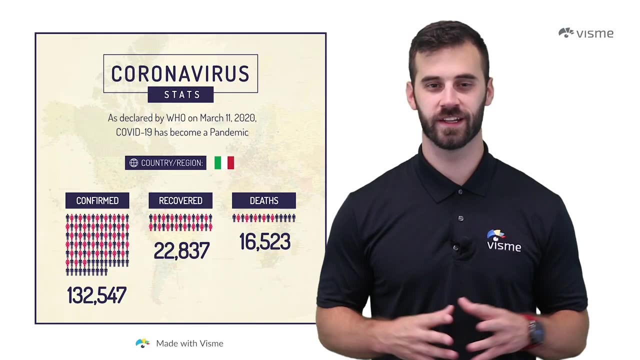 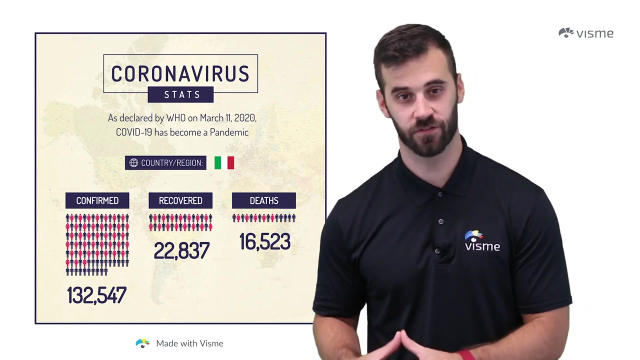 and more. Get out your pen and paper and let's begin, shall we? Let's start with what data visualization is. While the term sounds scary, a data visualization is meant to make understanding information easier. It's just a graphical representation of data. 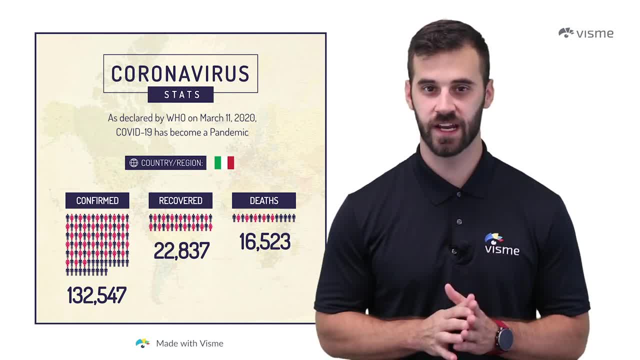 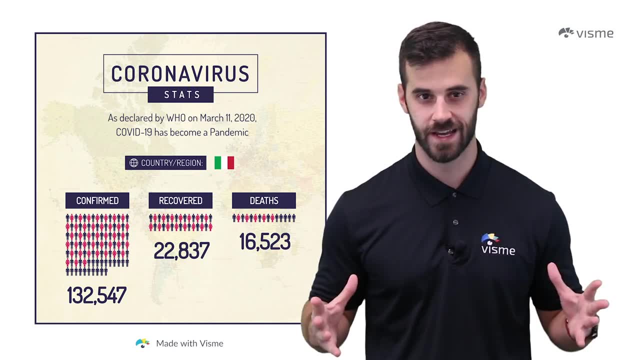 Rather than presenting data in a complex spreadsheet, you can create an image that will illustrate the information in a simpler way. Viewers don't have to scour a fact sheet looking for the story. They can easily scan and quickly find what they're looking for. 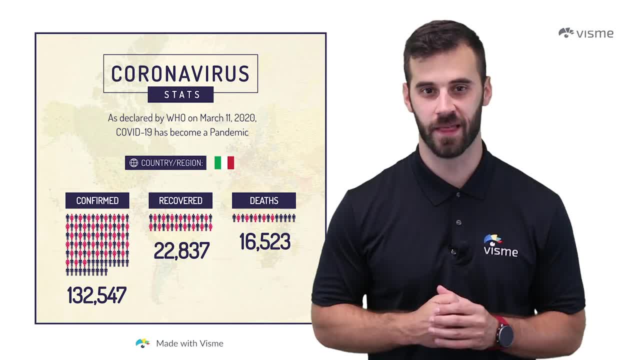 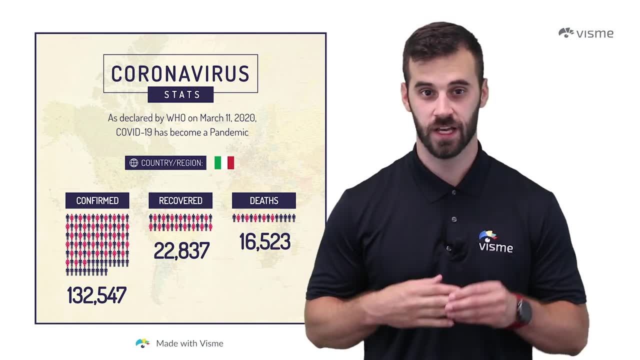 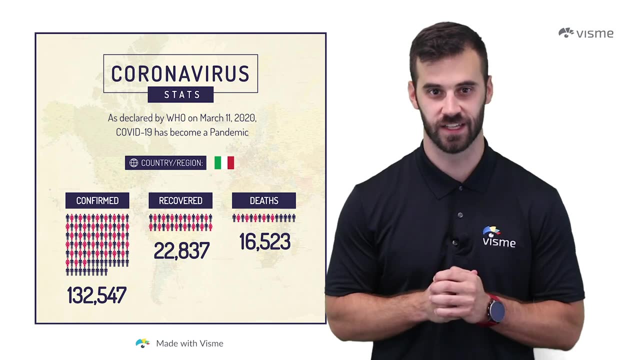 And you don't have to be a data genius to create them. Anyone and everyone can create them, no matter their profession. Marketers, teachers, healthcare professionals- consider this infographic here. Your profession is not an excuse to not create data visualizations You can create. 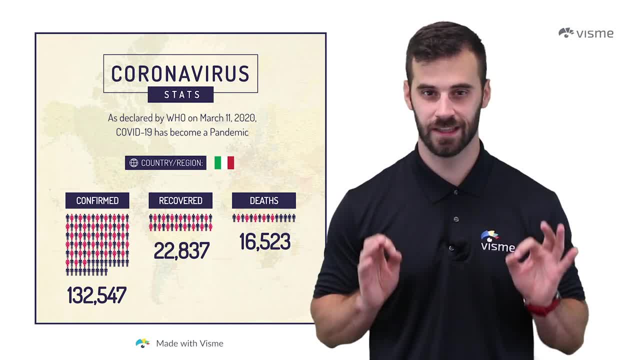 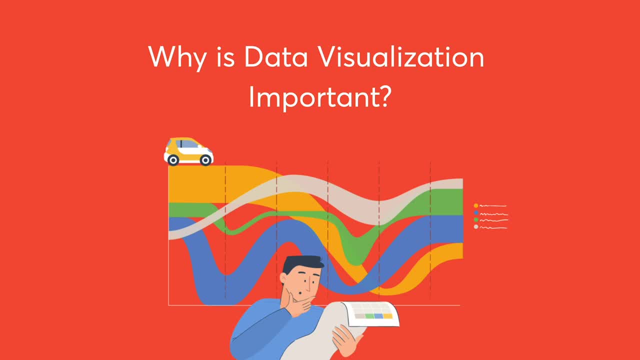 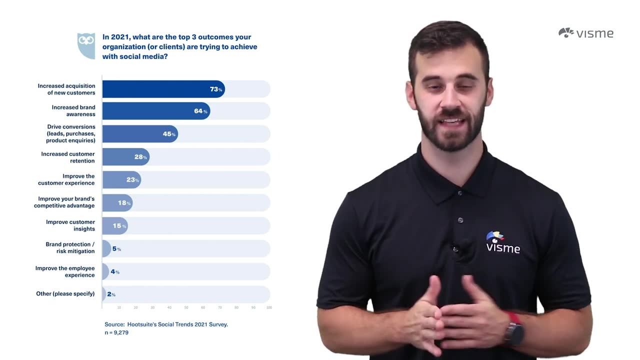 so much value for your audience by spending just a little bit of extra time building them I just mentioned. As I mentioned creating value for your audience, let's dive into four ways of doing so. The first reason is how easy it makes data to digest. 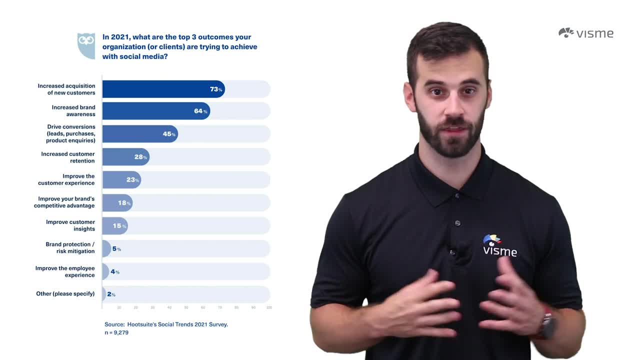 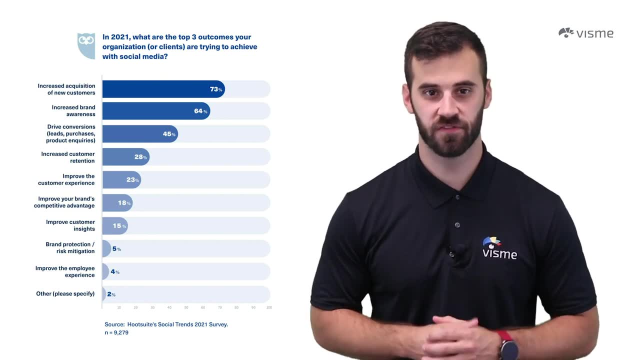 You can write a full report if you'd like, and hope that your audience reads it all the way through to understand your point. or you can create an infographic like this, which is still somewhat complex but simplifies the information in an easy to understand manner. 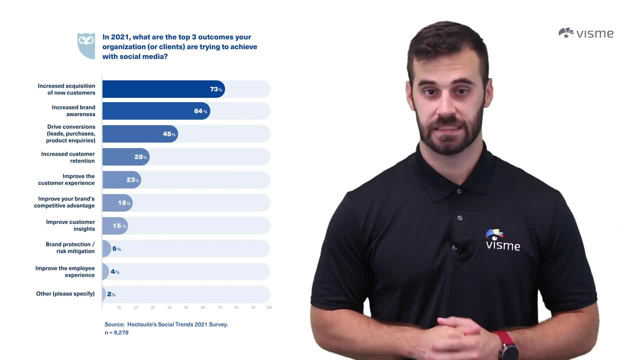 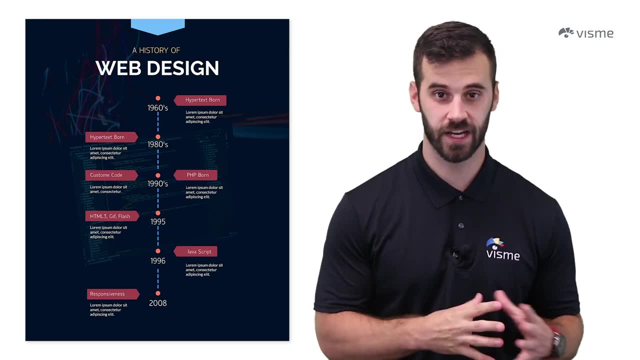 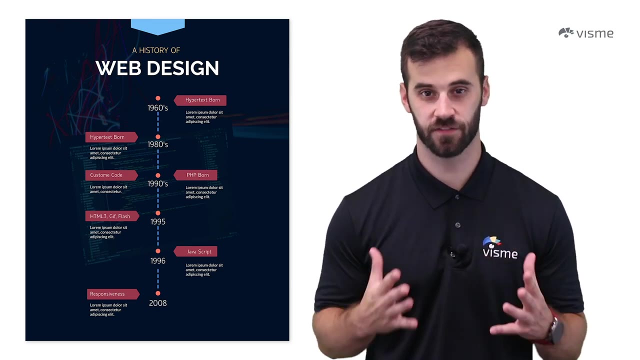 Imagine if all of this was written in paragraph form. yikes. The second reason is the ability to discover patterns easier. Trends emerge from data over time and if you monitor that data through graphics, they're much easier to notice. Scatter plots or charts can help you identify them and then, once you do, present them with. 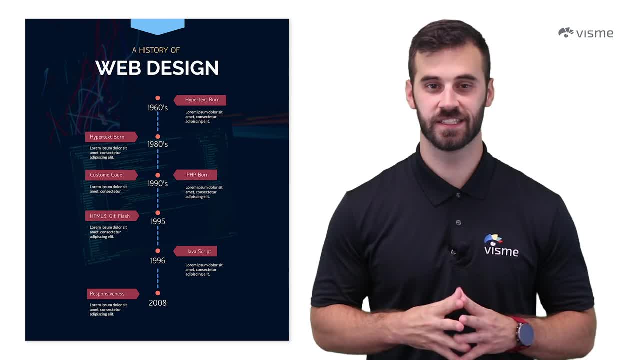 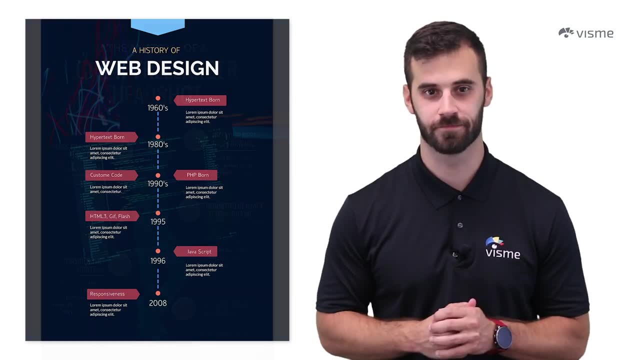 an infographic similar to this one. I haven't mentioned this yet, but all of the examples you'll see in this video are templates you can edit in VisMe right now, so keep them in mind. If you've been learning or gathering information for a long period of time, you might want. 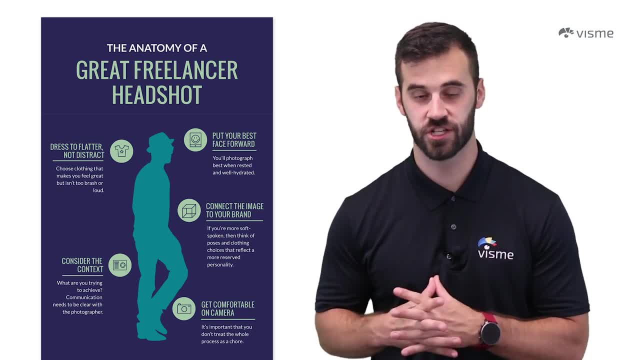 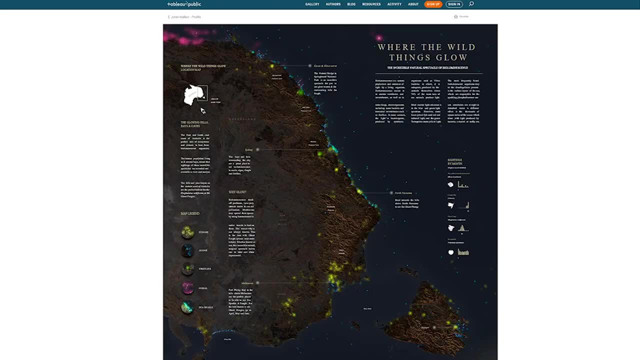 to use a data visualization to help you compile that information into one place. It's more engaging and an image is always easier to remember than text alone, Which is our fourth reason. The visual nature of a data visualization helps viewers understand and remember it better. 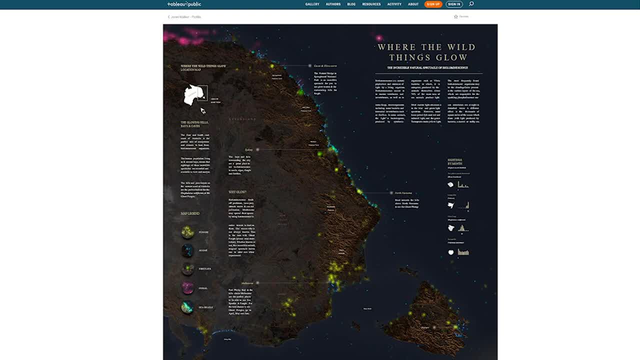 They'll soak in that image like a sponge and will be able to recall the information that went with it. This is a detailed infographic about bioluminescence in Australia. The geographical image makes it easier to remember. It's a good way to remember where it's present and where it's not along Australia's eastern. 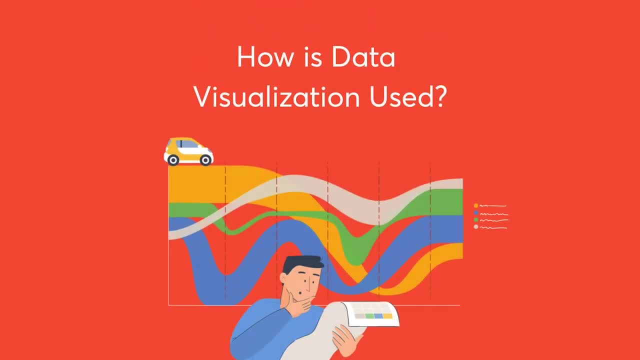 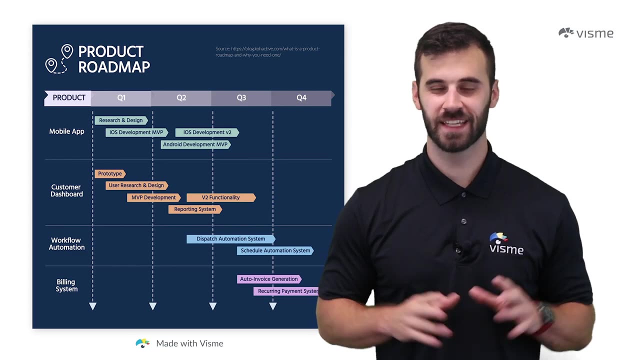 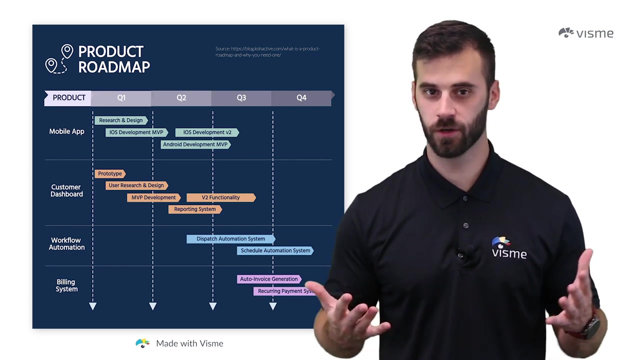 coast. All right, we have our feet wet in the data visualization pond. Let's get a little bit deeper now and explore five ways data visualization can be used. One is to plan schedules. Are you familiar with Google Calendar? Well, that's become a data visualization. 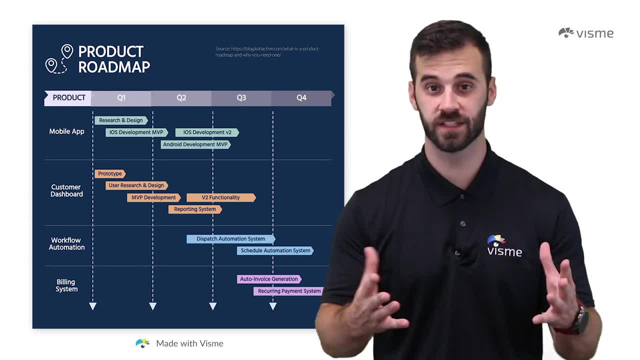 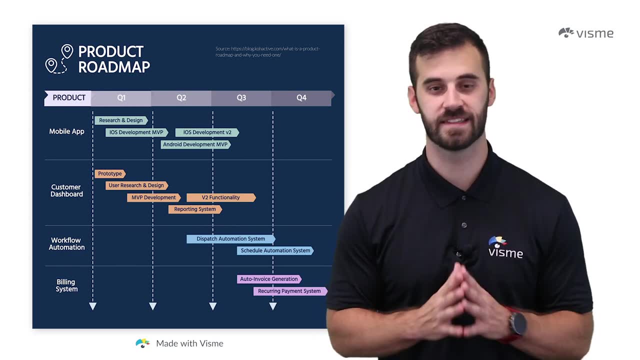 You can lay out a timeline or project plan for your days or months, Whether through Google or on your own. If you're on deadline, a visualization showing what needs to happen before the big day is a great idea. I suggest starting at the end and working backwards. 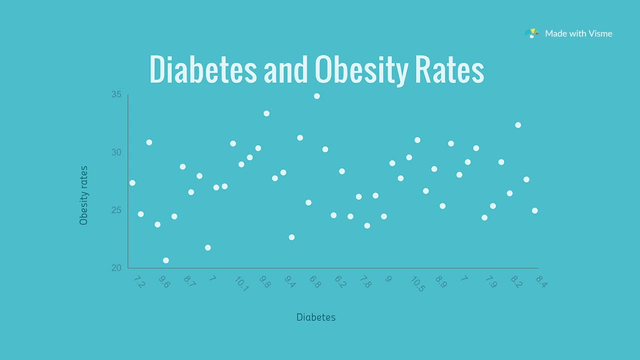 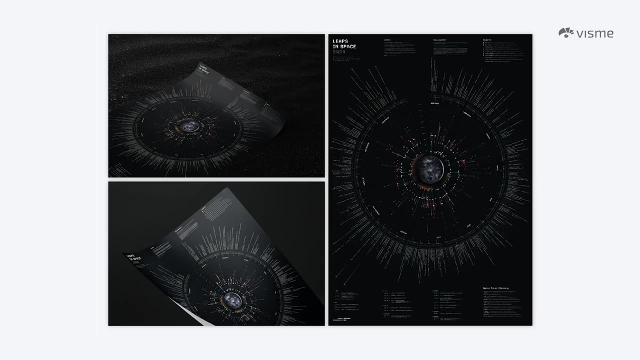 Another way data visualization is used is to pinpoint relationships. How are two or more things related? This is when a scatterplot becomes your new best friend. If time is one of the variables in your data, a graphic can help share changes over that time period. 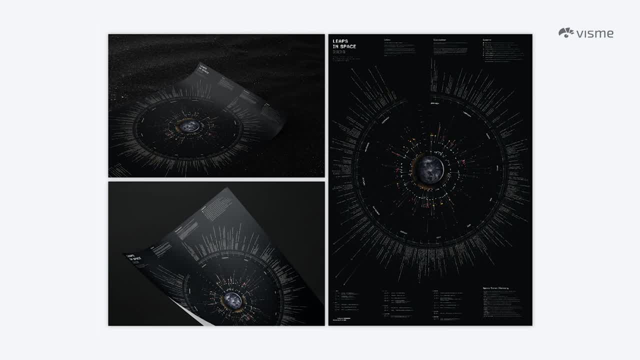 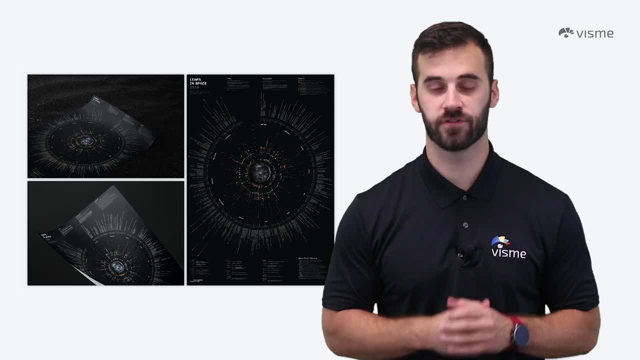 By recognizing the trends from the past, You're going to be able to plan your day. Your data visualization will help you predict what outcomes to expect in the future. Frequency falls in line with predictive ability as well. After you've compiled so much data, you'll have an idea of the frequency you can expect. 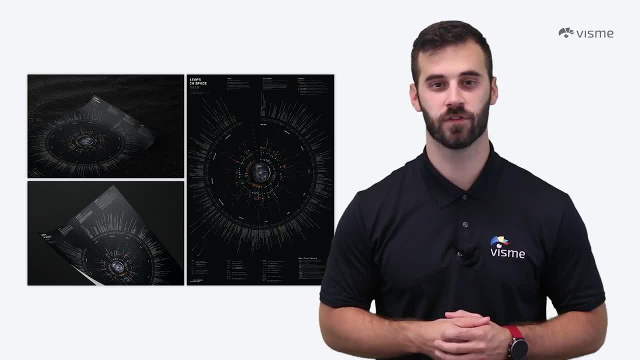 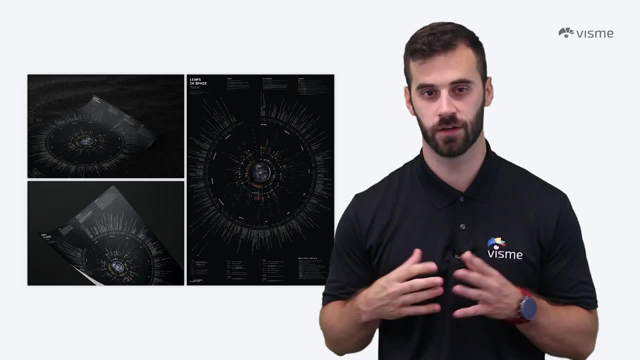 something. This will require a lot of research, but will be helpful for both yourself and your viewers And our last. way that data visualizations are typically used is to interpret value and risk. Rather than sorting through pages of information, a simple data visualization can help you assess. 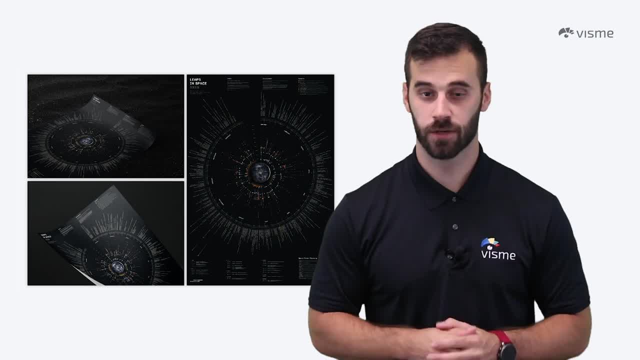 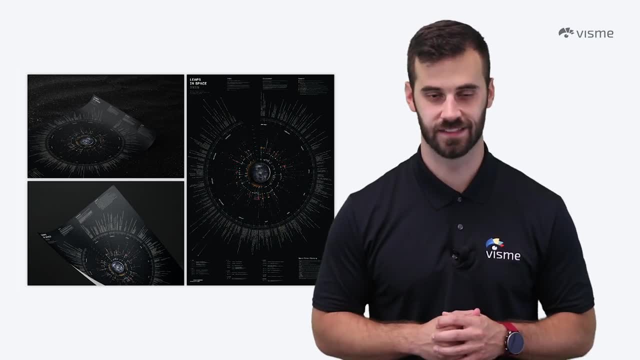 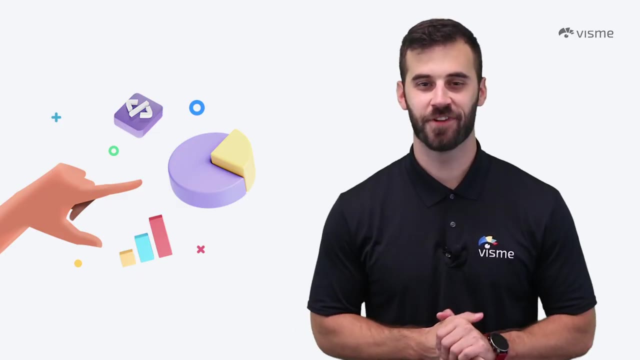 the situation and determine if taking action is necessary. Your brain can process multiple variables much more easily in an infographic than it can in a page full of text. All right, you've heard me touch on various types of data visualizations already. To halt any confusion and answer any questions, let's touch on some of the most popular. 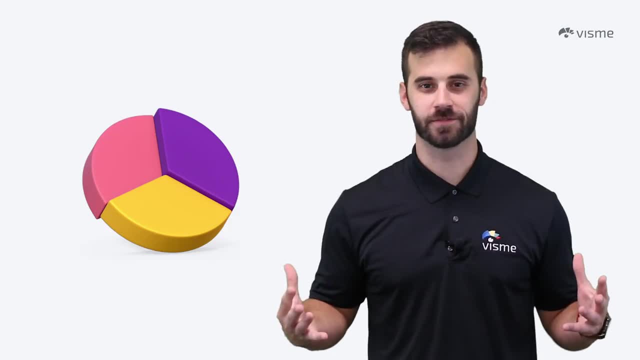 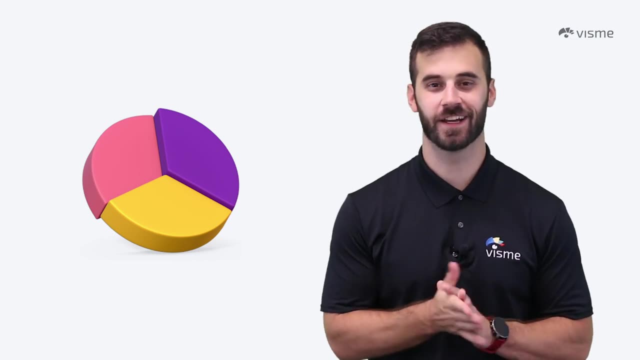 Let's start with graphs. Let me preface this by saying there are dozens of graphs you can choose from. For the sake of this video, I'm only going to share a couple of the most popular. Pie charts were our best friend in third grade. 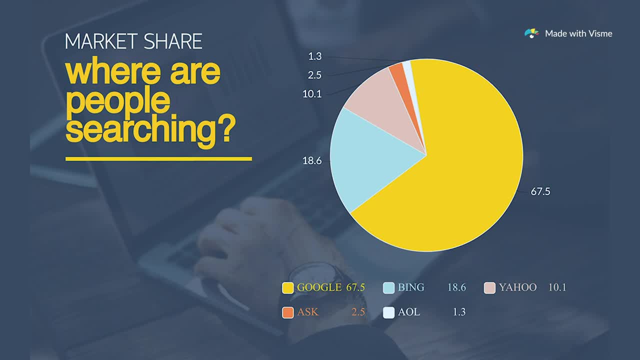 And well, you should read them. You can connect after all these years. If you have seven or less percentage points and their differences in value are wide, use a pie chart. They're simple and everyone understands them. Bar charts are another good example for easily understood data visualizations. 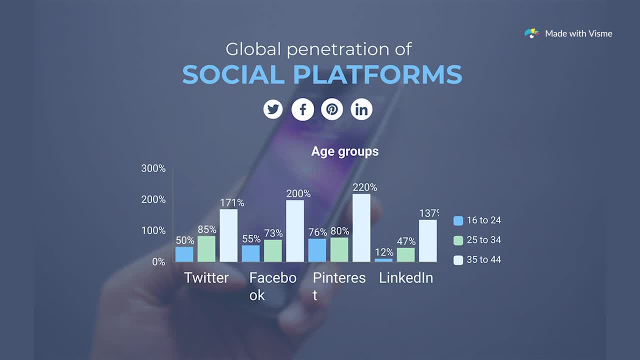 They mostly speak for themselves and I'm sure you've seen them before. Again, if you're thinking there's no way you can create these, Visme has your back. This is a template right here that you can edit to fit your data right now at vismecom. 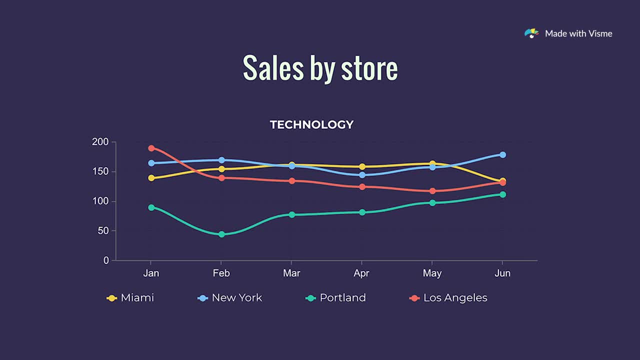 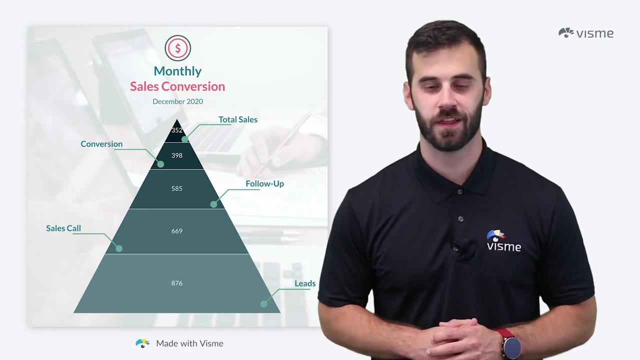 Pie charts take one fixed value and however many variables and place them adjacent to one another. These are perfect to discover trends or to see how one variable may be superior or inferior to another. Three prominent charts that you can use include pyramid charts, stacked area charts and radar. 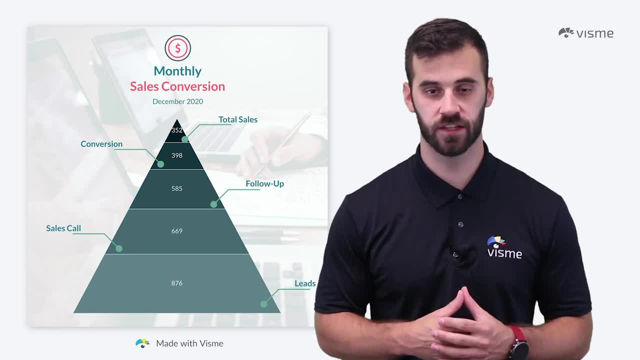 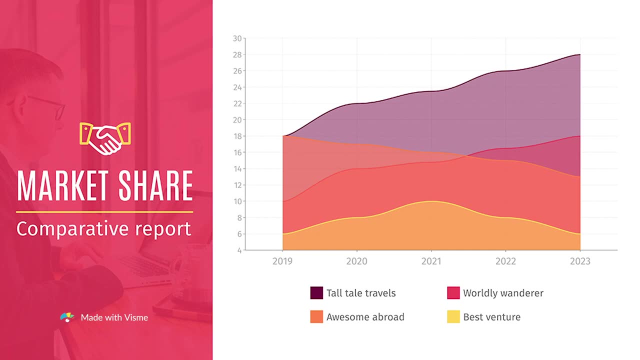 charts. Pyramid charts showcase visual hierarchy. They can illustrate income importance or the difference between your income and your wealth. They can also show the difference between leads and actual sales. as we see here, Stacked area charts are similar to your line charts. 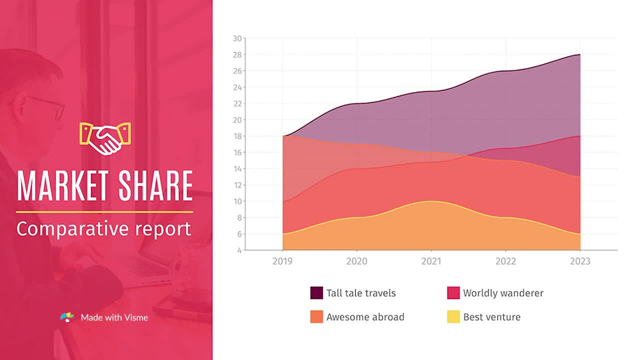 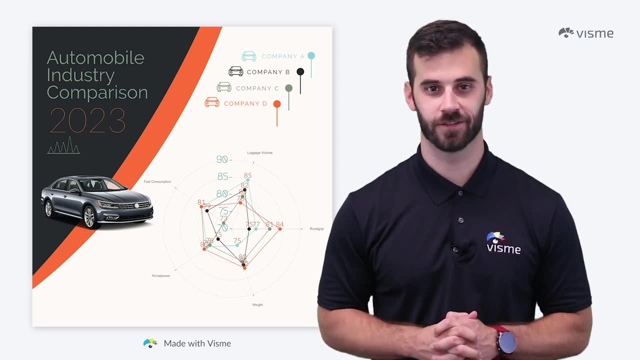 They'll visualize changes over different values over time. There's not one fixed variable here. And the last chart I want to put on your radar is the radar chart. You may have also heard of these by the name of spider or web charts, but it looks something. 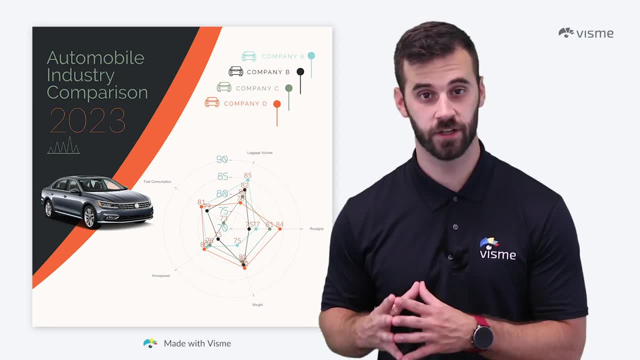 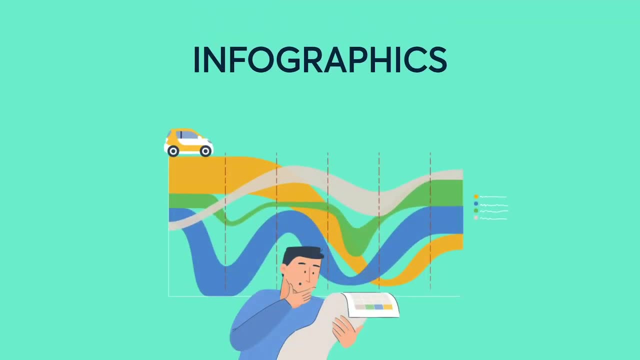 like this. They're great for identifying if something is well-rounded or maybe lacking in one specific area against other competition. You can also use them to visualize your income and your wealth. Infographics rely on text a bit more than a standard data visualization. 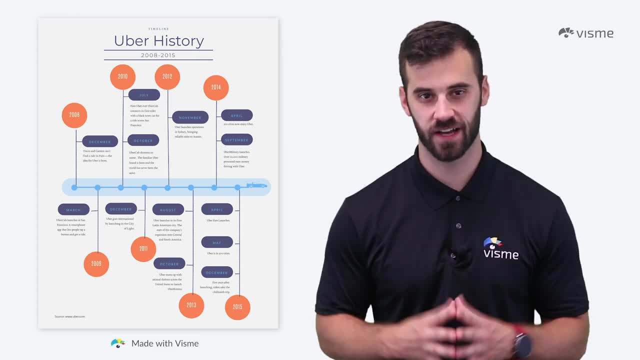 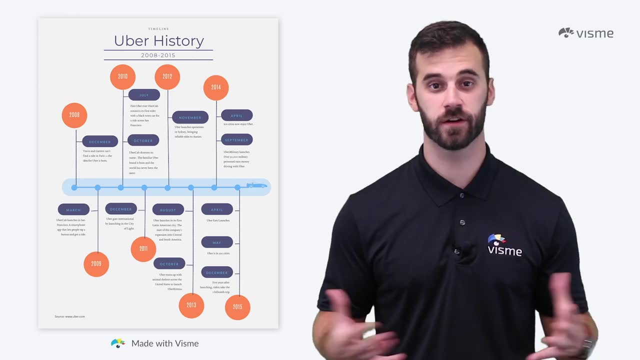 It's still kept to a minimum, but it might be necessary depending on the type of infographic. One example is a timeline infographic. These will have some text, but you can follow along easier, knowing exactly when events were taking place, by actually seeing it along the timeline. 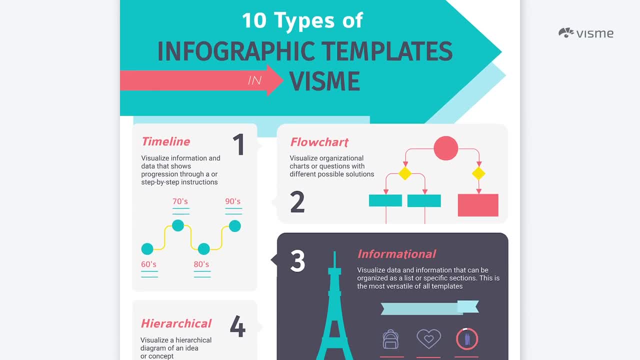 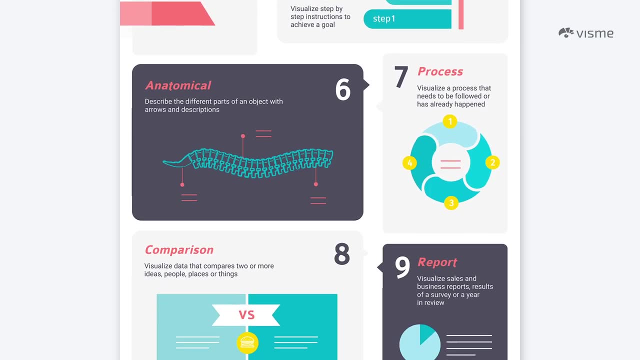 An informational infographic will carry a lot more text and may even feature multiple data visualizations all in one graphic. You'll want icons, colors and charts, but don't overload the graphic and make it too overwhelming. Keep it organized like we see with this FISME template. 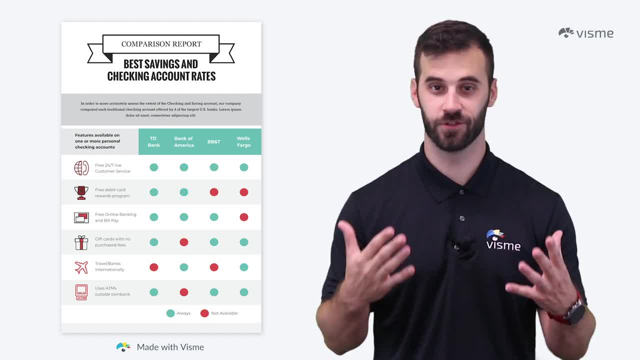 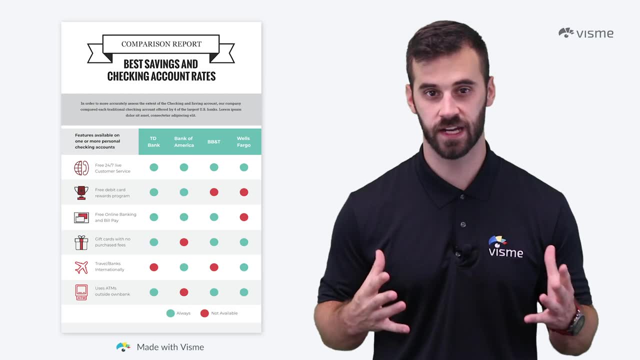 And while there's plenty more infographics to check out, which I encourage you to do so, for the sake of time I just want to touch on comparison infographics. This is for side-by-side comparisons of data, helping you or your audience make informed. 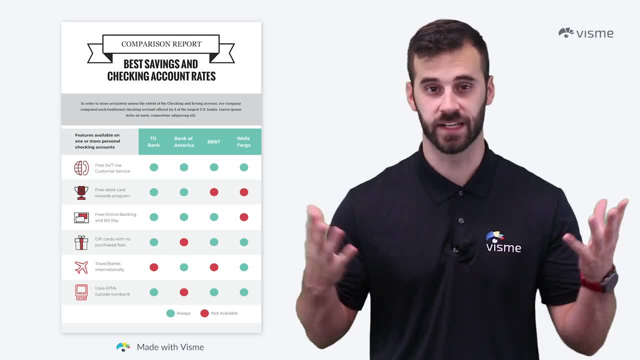 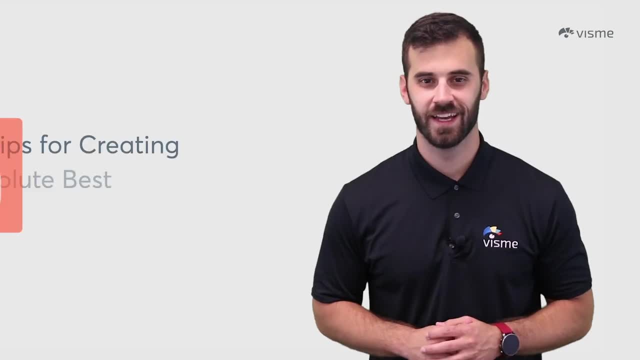 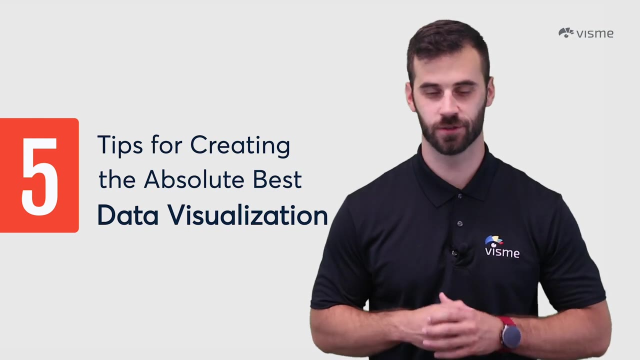 decisions. They're great for comparing cars, homes or banks. Let's see here. As we near the end of this video, I want to leave you with five tips for creating the absolute best data visualization that you can. First, know your audience. 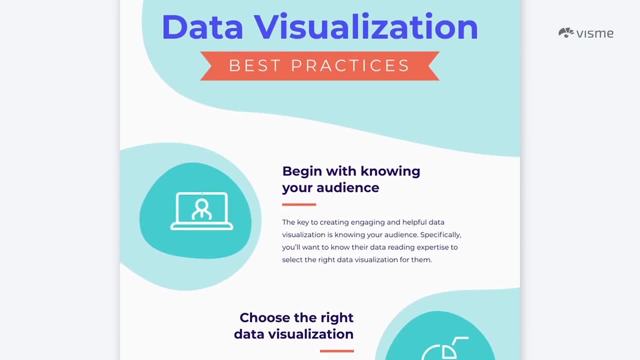 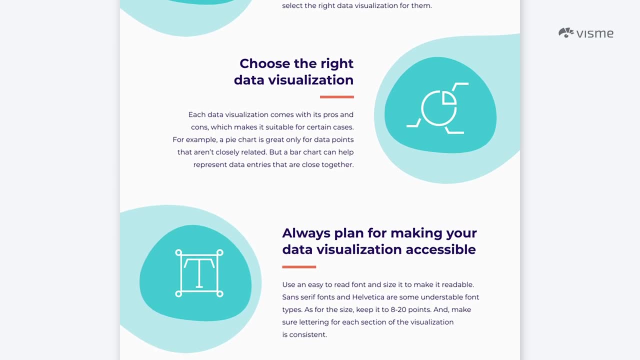 Understand their knowledge and if they'll be able to comprehend a complex visual or if you'll need to simplify it. Are you talking to high schoolers or experienced professionals, or are you presenting a spider chart to your HR department? Let me know in the comments. 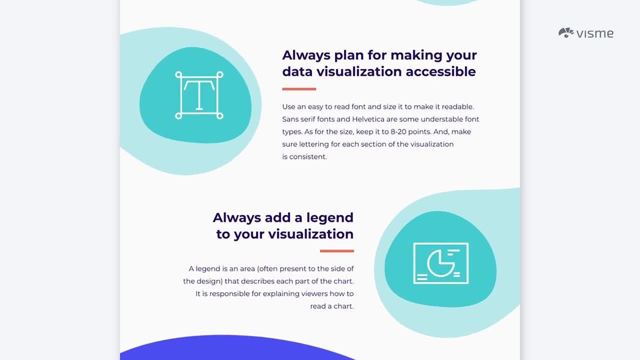 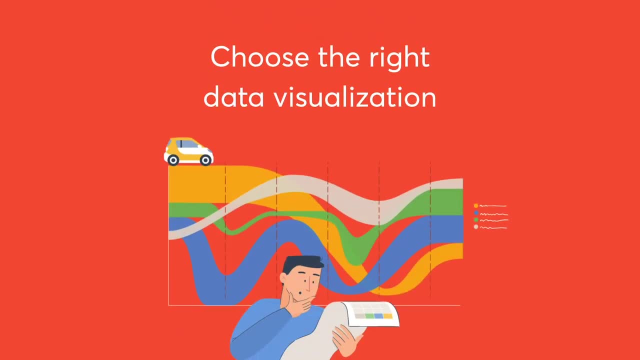 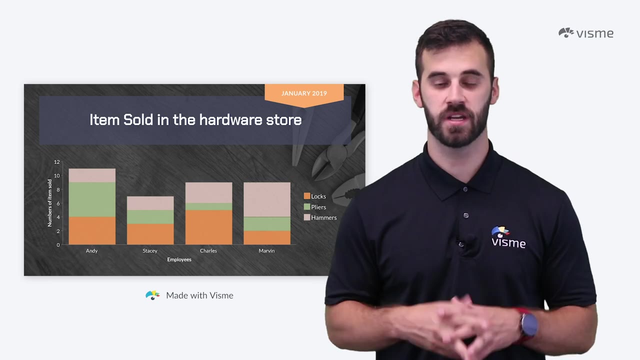 The HR department will recognize it right away because they have more experience with it. Communications may not. That's another reason why you need to choose the right data visualization. As I mentioned, a pie chart would not be great for data points that are very similar. 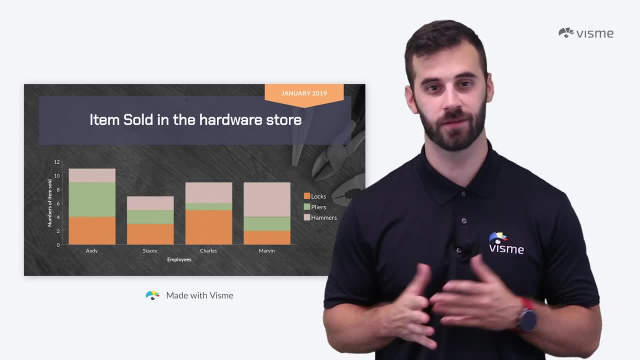 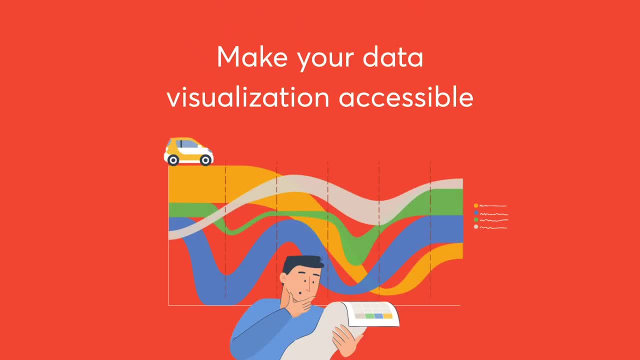 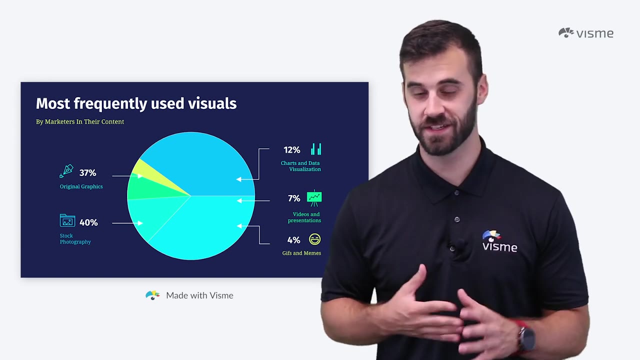 That's when you'd want a bar chart. A stacked bar chart is good for comparing maybe two to three variables, but any more than that. A comparison chart becomes your friend. Some quick design tips for you. If you follow our channel, you've probably heard me say these before. but don't use 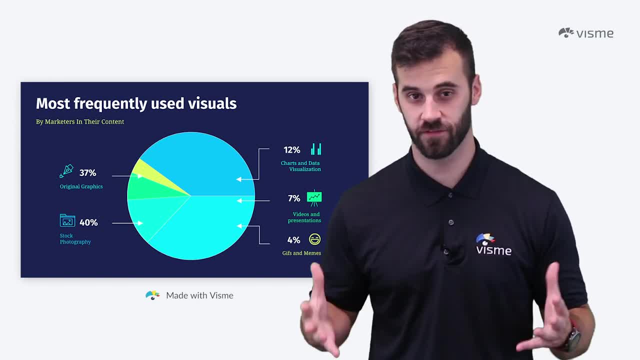 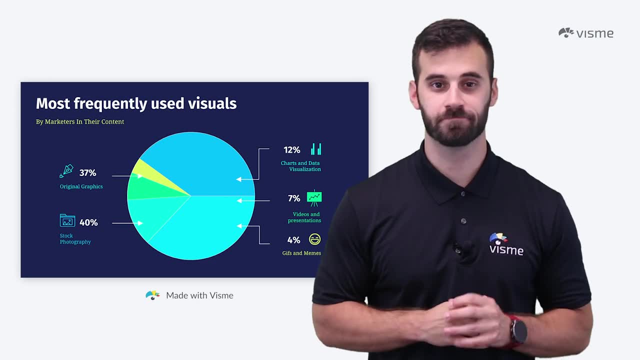 more than three fonts. Keep the sizing to between eight and 20 point fonts. Select colors that are easy on the eyes and complement each other well. Pro tip: blue and purple, green and brown, blue and gray. and green and gray are combos. 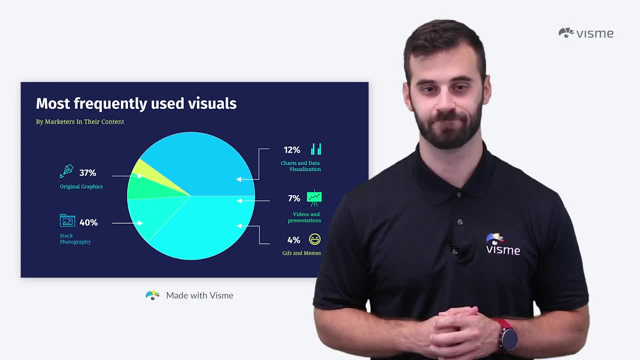 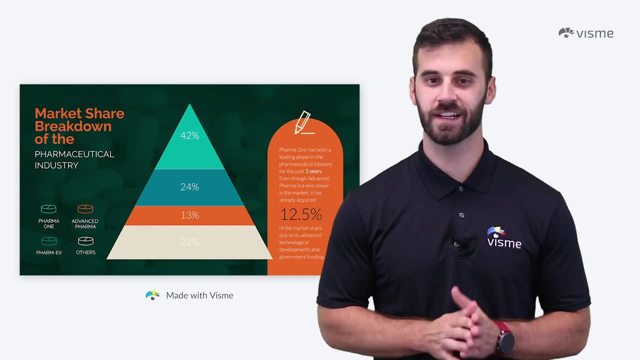 that colorblind people can't make out, So keep that in mind. When a viewer reads a chart, they may need a legend to help them understand what exactly they're looking at. A legend is what will tell them how to read the chart.